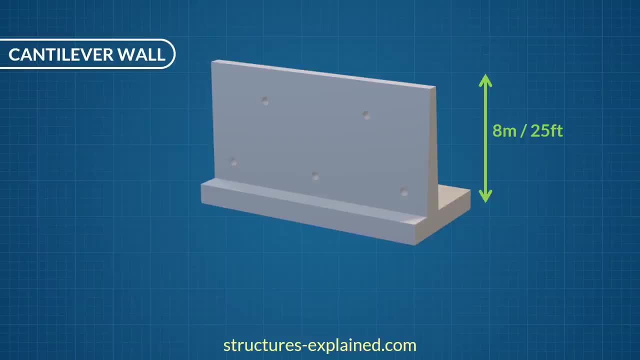 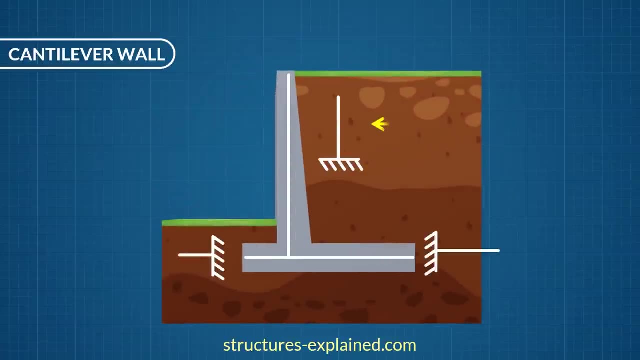 ft. The three components, which are stem, toe and heel, act as one way cantilever slabs. The stem acts as vertical cantilever under lateral earth pressure, The heel acts as a vertical cantilever under the action of net weight of retained earth and the toe acts as a cantilever under the action. 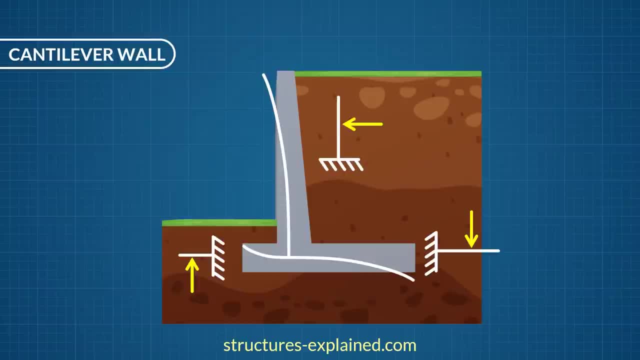 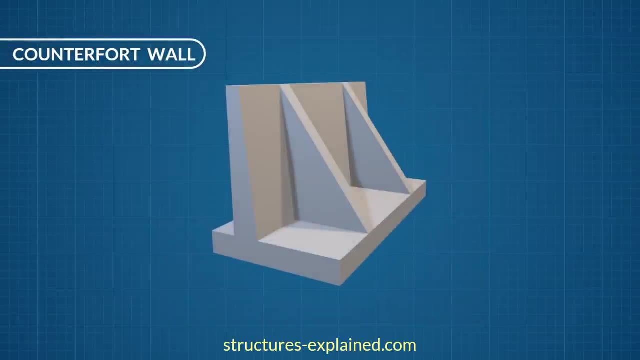 of net soil pressure. Hence the resulting deformed shape would look something like this: The main reinforcement resisting the tension forces will be provided in these regions, as the concrete is weak in tension. Third type of retaining wall is a counterfort wall. Such type of walls have supports. 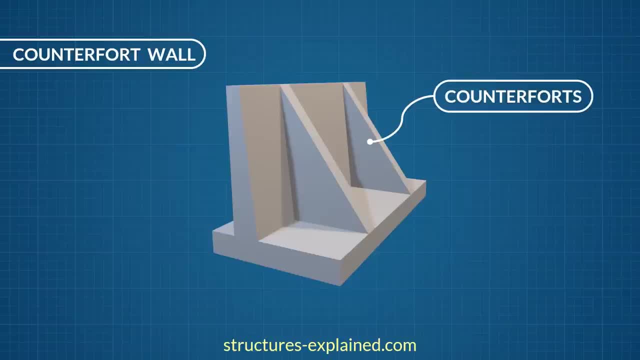 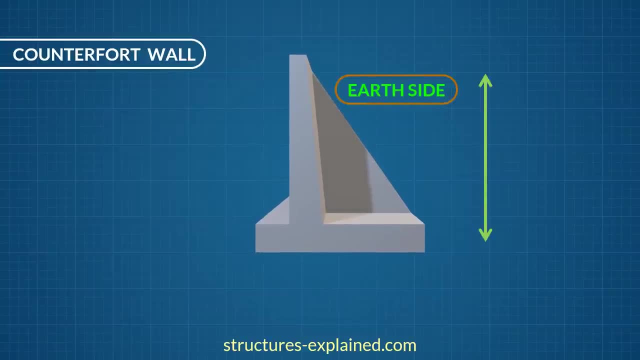 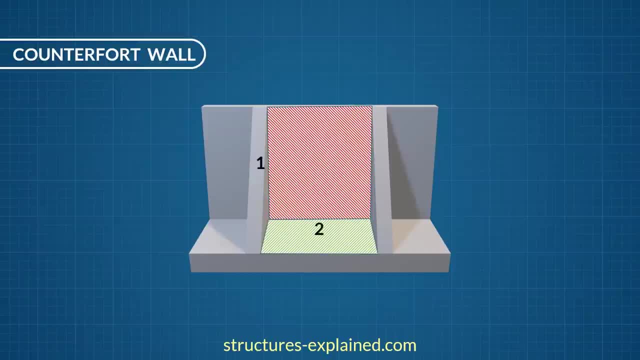 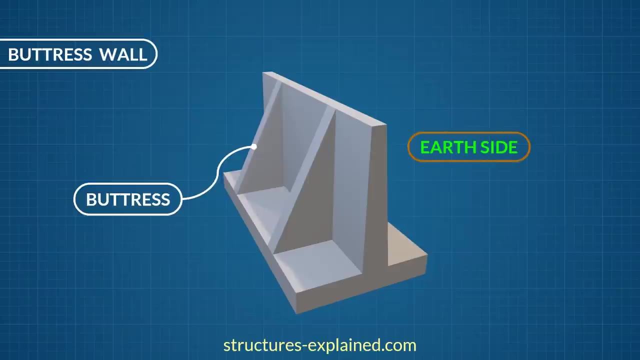 The counterforts subdivide the stem and heel into rectangular panels. These panels are now supported on three sides and free at one edge. Fourth type of retaining wall is a buttress wall, which is similar to the counterfort wall, but the supports are are now on the toe side and not buried in the earth. 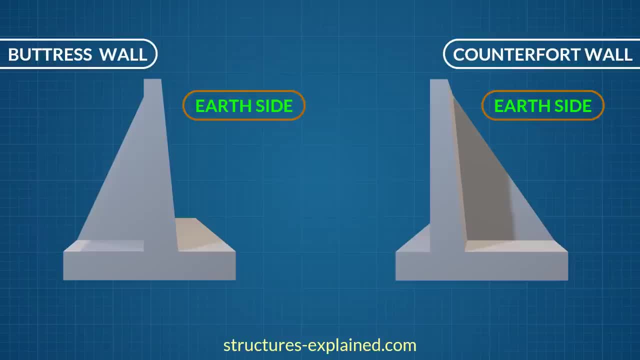 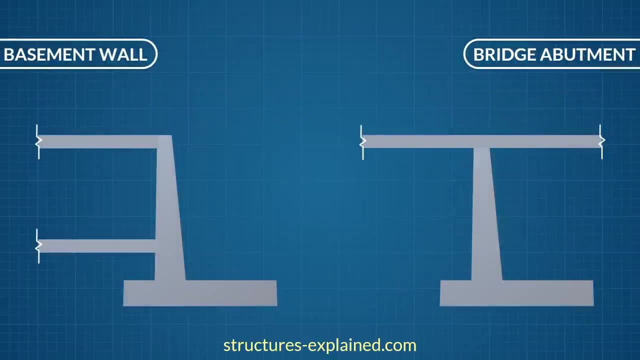 Between the two counter fort and buttress. counter fort wall is preferred, as it provides usable space in front of the wall and looks clean. In terms of efficiency and economy, buttress wall is preferred. Fifth type of retaining wall is restrained on the top and can be found in buildings as 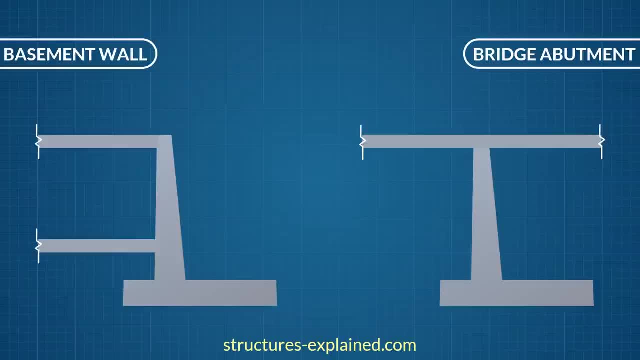 basement walls and in bridges as abutments. In both these cases the stem is supported by floor slab in buildings and deck in bridges. For the analysis part, the stem is considered as a beam fixed at the base and simply supported or partially restrained at the top. 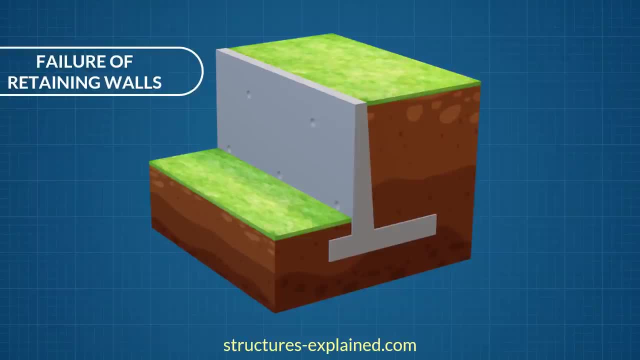 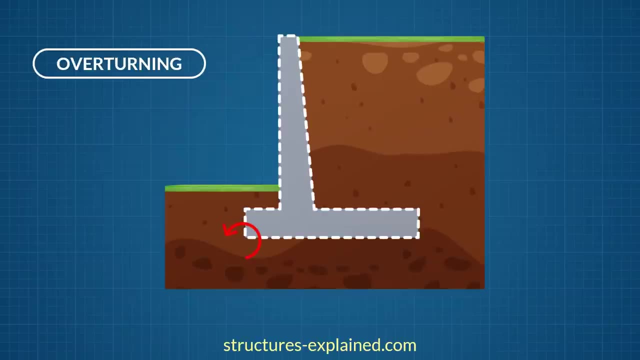 Now let's understand the failure modes of a cantilever retaining wall. First is failure by overturning. In this failure mode, the toe will act as center of rotation and the wall would deform something like this: In absence of toe, the footing base below the stem will act as center of rotation. 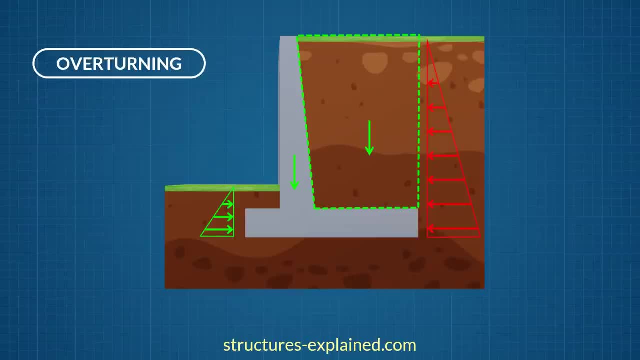 All the lateral pressures will act as overturning forces, while the weight of the wall and soil on the heel will act as stabilizing forces. Second kind of failure is by sliding. All lateral forces try to slide the wall. The resistance against sliding is mainly provided by the friction between base slab and the 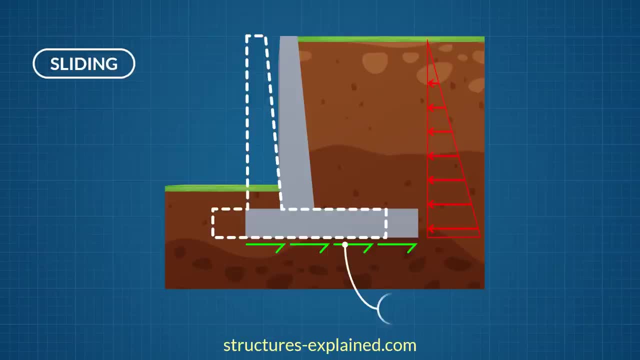 soil below it. The frictional force is given by µ times r. where µ is the static force, The friction between the base slab and the soil below it is given by µ times r. where µ is the static force, The friction between the base slab and the soil below it is given: 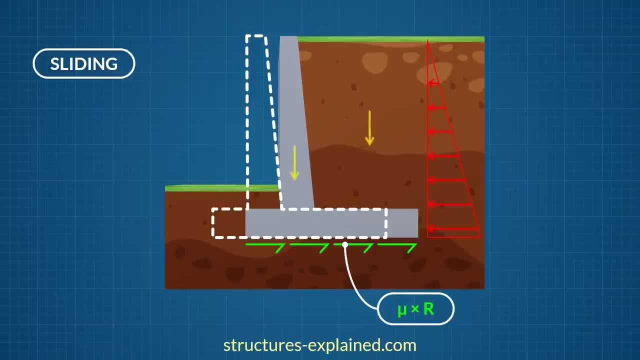 by µ times r, where µ is the static friction coefficient between soil and concrete and r is the resultant soil pressure. When the lateral pressures are high and wall fails in sliding, a shear key can be introduced to increase the sliding resistance. The position of shear key is decided in such a way that the flexural reinforcement from 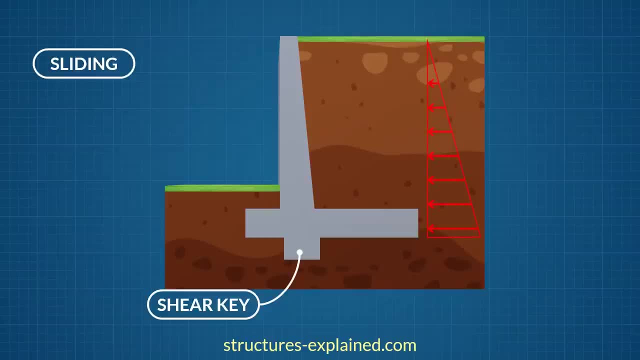 stem can be extended straight into the shear key and it can create maximum counter pressure. The pressure generated on shear key resists the lateral forces. Third kind of failure occurs when the soil below the wall fails in bearing pressure. A soil can bear a certain amount of allowable pressure, which is found by a geotechnical study. 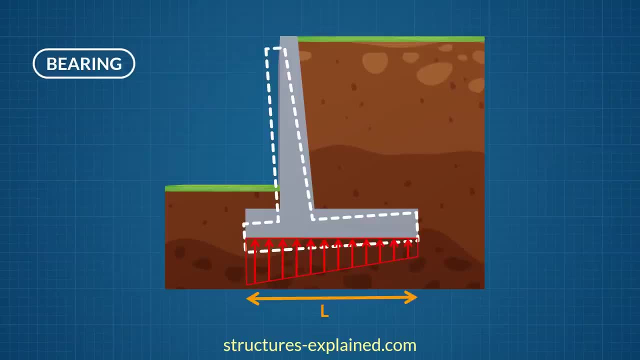 Hence the width L of the base slab must be adequate to distribute the vertical reaction. Now let us see the forces which act on a simple cantilever retaining wall. First, let's assume a flat backfill, with no additional load. The soil will apply lateral. 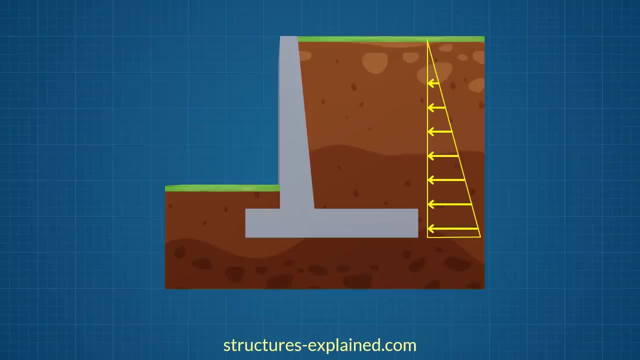 pressure, which will vary with the force applied. The force applied will be equal to the force applied on top of the wall. The force applied on top of the wall will vary with the depth of the soil, which means top of the wall will bear no pressure, while bottom of the wall 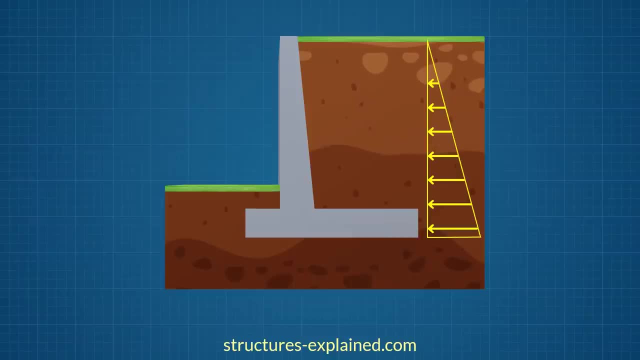 will bear maximum pressure. This pressure is called active pressure, or in short Pa, as it is actively trying to push the wall along it. The intensity of pressure at bottom will be Ka times gamma s times h. In this expression, h is the total height of the backfill, gamma is the unit weight of the soil. Here Ka is. 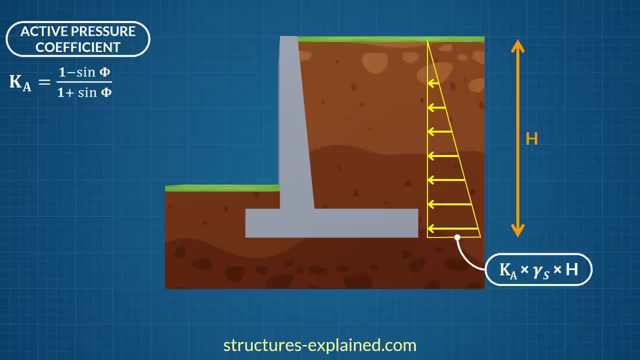 the pressure coefficient based on the Rankine's theory and is calculated via this expression. Here, angle phi is the angle of shearing resistance or angle of repose for the soil When the backfill is sloped. the expression changes to this where additional angle theta is the 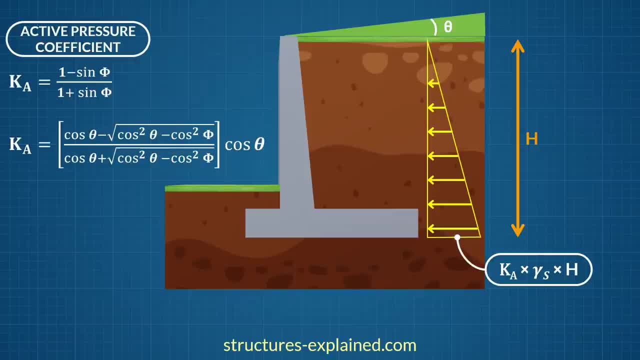 angle of inclination of the backfill For a typical granular soil such as sand phi is 30 degrees, which makes Ka as 1 by 3.. This pressure Pa will be equal to the angle of the backfill. The angle of the backfill will be equal to the angle of the backfill For a typical granular 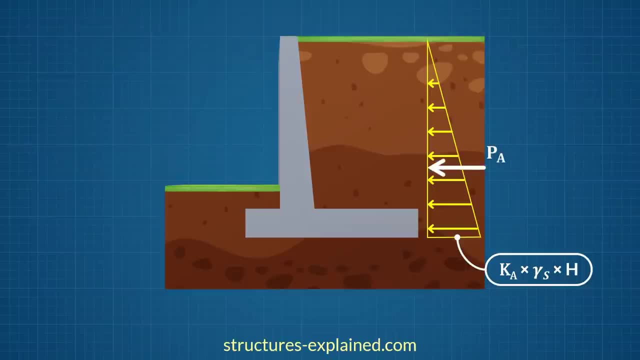 soil such as sand phi, is 30 degrees, which makes Ka as 1 by 3.. This pressure Pa, will be equal to the angle of the backfill. The angle of the backfill will act at the centroid of the pressure intensity triangle, which is at a distance of h by 3 from the base. The value of this force will be area. 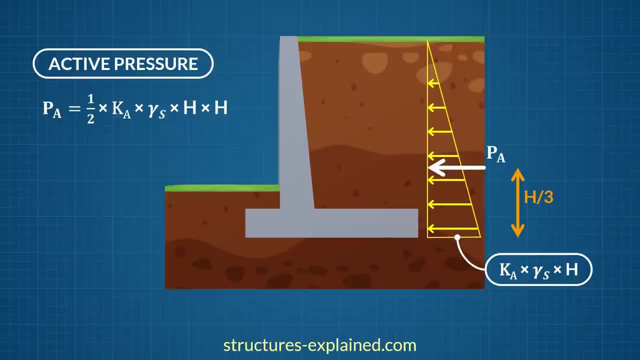 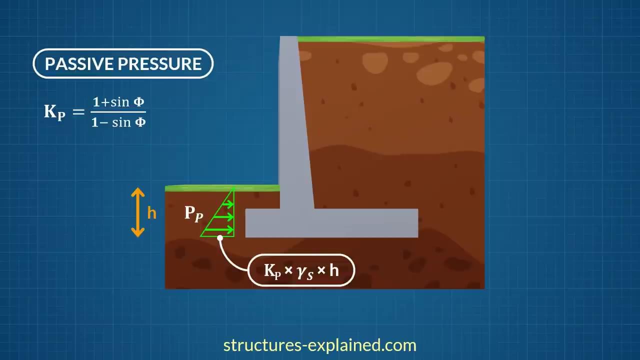 of triangle which is half times base into height. This was about the active pressure. There is one more pressure, which is called as passive pressure, which acts from the toe side and helps the retaining wall. The coefficient of passive pressure, Kp, is calculated by this expression, which comes out to be 3 for granular. 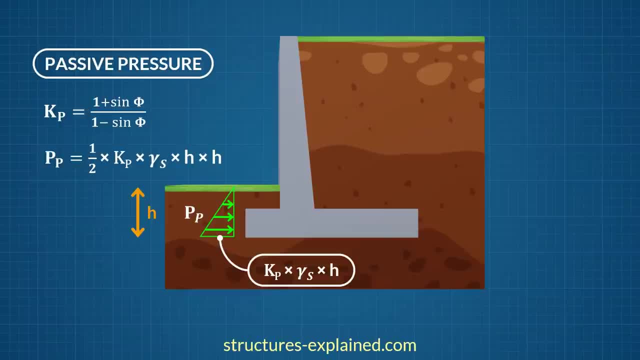 soil of 30 degrees. This pressure is generally not included in design calculations, hence making the design conservative. Next force which will act on the wall is the surcharge. if considered, This is also an active pressure. The surcharge load can come from various means, such as vehicular traffic or 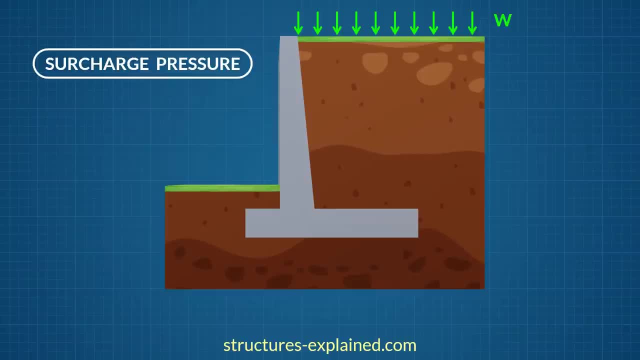 any other live loads. Let's consider surcharge having intensity of WN per m2 and uniformly distributed, This pressure will act laterally on the wall with an intensity of Ka times W. The force due to this surcharge is the area of rectangle, which is Ka times W times height. 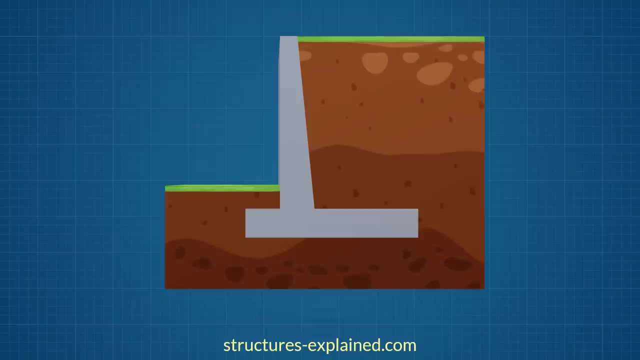 Next force which acts on the wall is from the water present behind it. This case is bit complex, so let's simplify it slowly. When water does not have an escape route, it will get accumulated and apply pressure on the wall. Let's consider the height till. 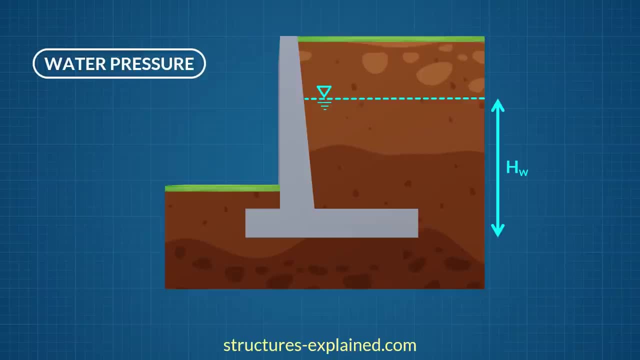 which the soil is submerged. This wall will act on the wall with an intensity of Ka times W. This pressure will act laterally on the wall with an intensity of Ka times W. The force in the water as hw. The remaining dry soil will have height of h-hw, where h is the total. 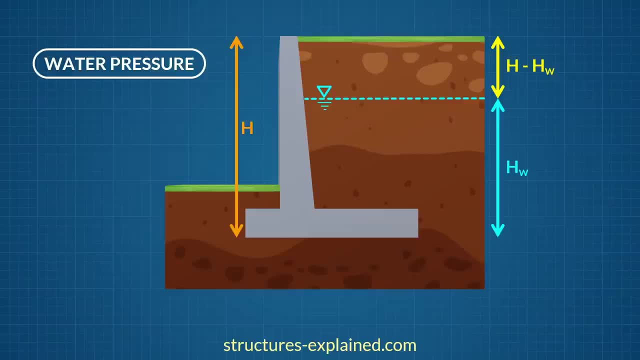 height. The dry soil will have a unit weight of γs and the submerged soil will have a unit weight of γsubmerged. Let's make the pressure diagram one by one. First will be the pressure from dry soil. let's call it Pa1.. This dry soil will act as surcharge for 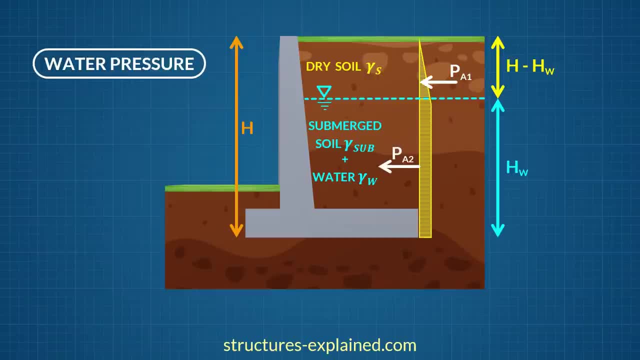 the remaining portion of the wall. Let's call this pressure Pa2.. The maximum intensity of the pressure will be Ka times unit weight of dry soil times dry soil height. Now let's talk about the submerged portion. Let the first pressure. let's call it Pa3.